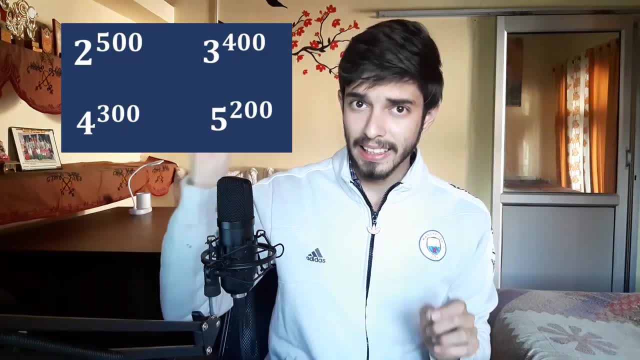 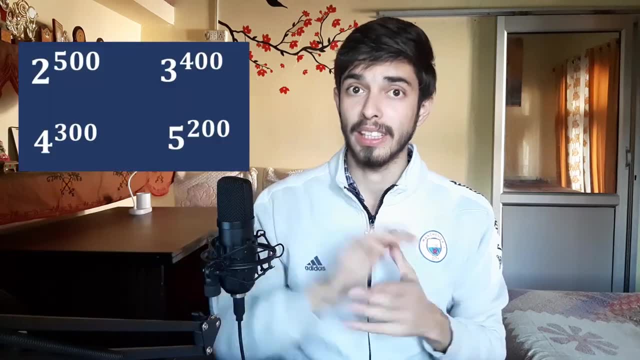 So let's come straight to the point. to solve any question like this, you just need to remember three rules, and that's it. with that, you can solve any kind of question like this one. Okay, so let us learn that. suppose there are two numbers, x and y. 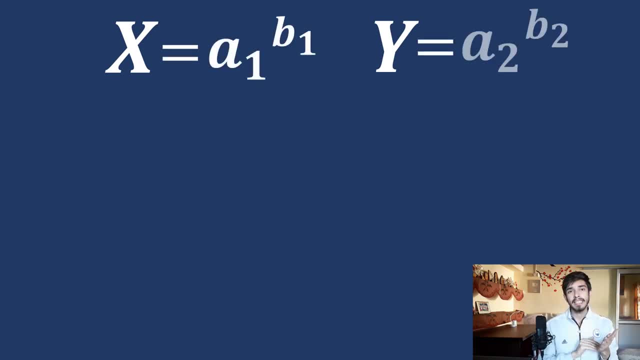 x is equal to a1 raised to the power b1, and y is equal to a2 raised to the power b2. now the three rules are as follows: x is greater than y if a1 is equal to a2 but b1 is greater than b2. for example, 3 raised to the power 6 is greater than 3 raised to the power 5. simple. 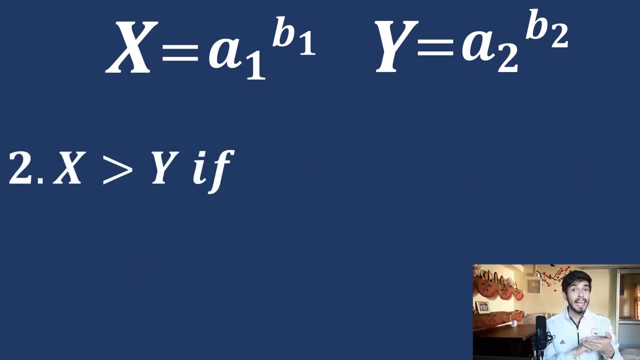 not very complicated now. the second rule is that x is greater than y. if a1 is greater than a2 and b1 is equal to b2, for example, 4 raised to the power 5 is greater than 3 raised to the power 5. 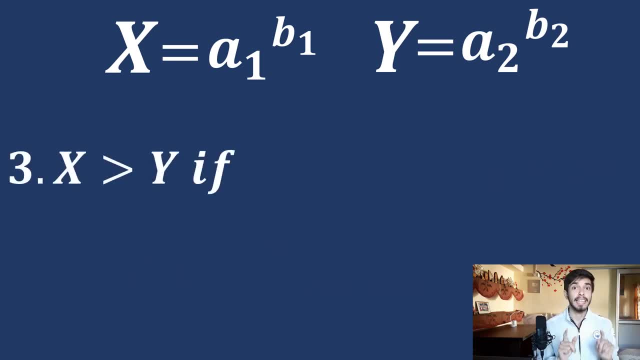 now. the third one is that x is greater than y. if a1 is greater than a2 and b1 is also greater than b2. for example, 4 raised to the power 5 will be greater than 3 raised to the power 4. so this is: 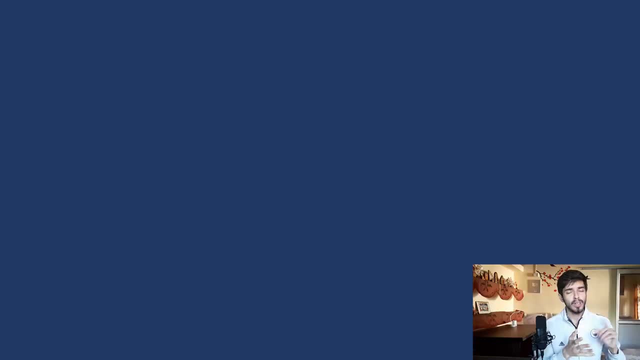 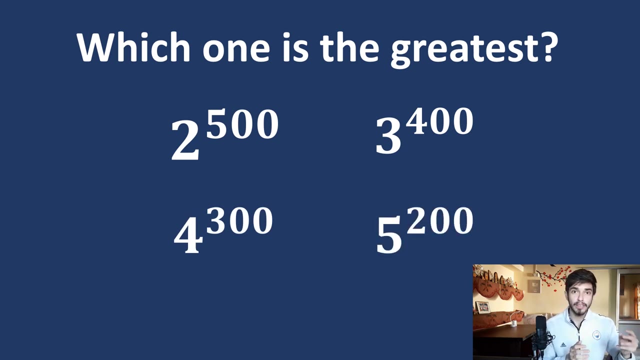 as simple as that. only these three simple rules. okay, so now let's come back to the question: which one is the greatest of the following numbers? see now, we won't calculate anything using the three rules. we will compare the powers and bases to find out the greatest one. now see in here. see 2 raised to the power, 500 and 4 raised to the power. 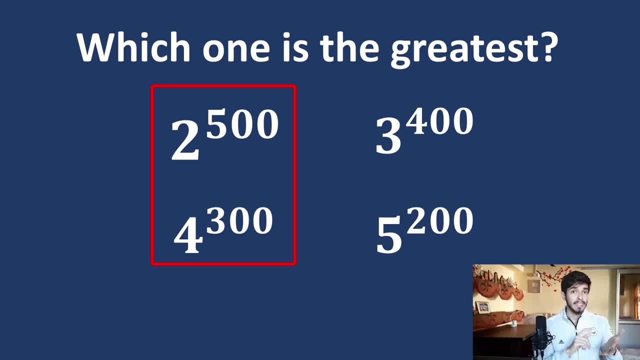 300 for these two. what we can do is this: see, there is 4, so 4 is basically 2 raised to the power 2, so we can write 4 as this. so it will become 2 raised to the power 500 and 2 raised to the power. 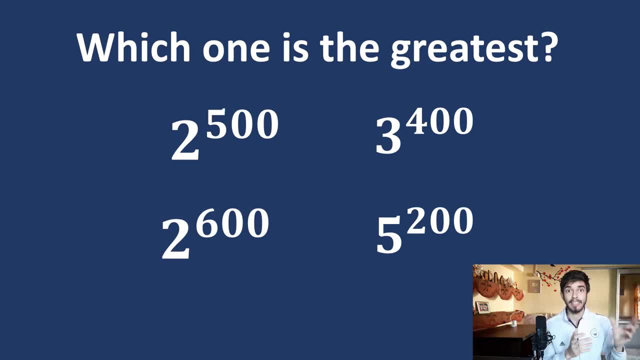 600. see, we just made the base equal to the power of 2 raised to the power 500 and 2 raised to the power 600, so that we can compare. so now it's simple. see, 600 is greater than 500. so, using the rule number,